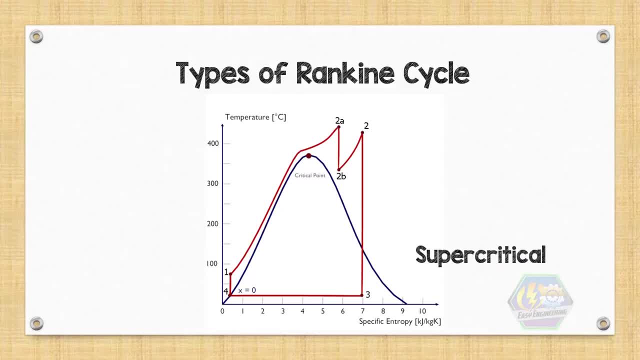 A supercritical Rankine Cycle is also one of the types, Just like reheat and regenerative Rankine Cycle. water is the working fluid, but it is operated at above its critical pressure. So those are the types of Rankine Cycle. 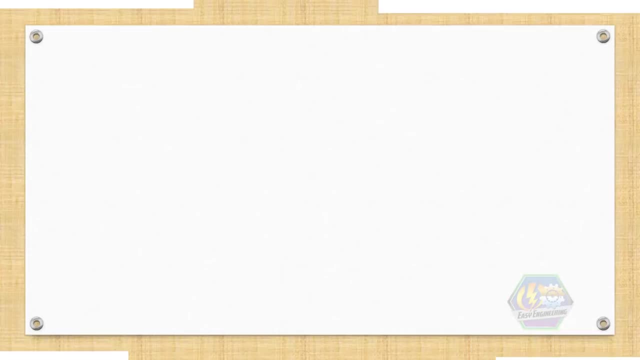 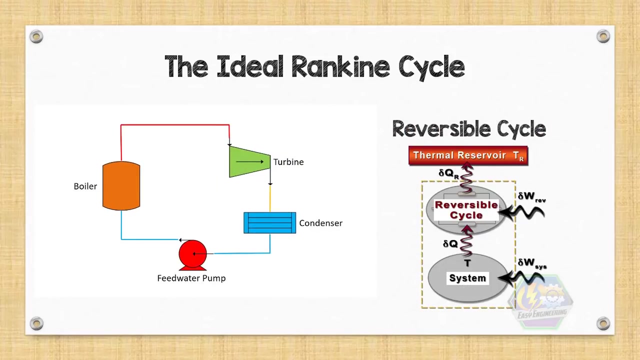 But here on this video, we will only discuss the most basic and fundamental of the cycle, The ideal Rankine Cycle. We must be aware first that this operates slightly different than the real Rankine Cycle. This is a reversible cycle. Common source of irreversibilities are neglected, such as frictional pressure drops and undesired heat transfer with the surroundings. 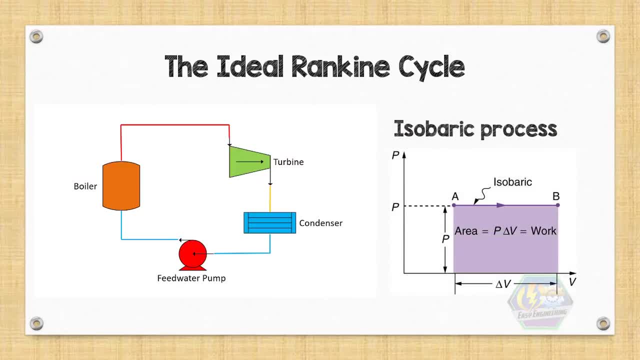 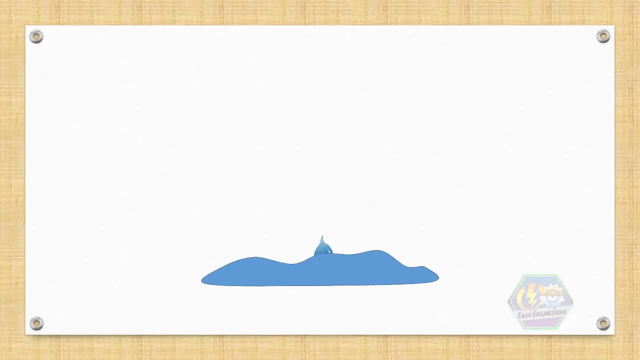 A constant pressure, or isobaric process, and constant entropy, or isentropic process are used for the equipments involved in the cycle. The working fluid is water and it will undergo a closed loop and will be reused constantly, So why do we use water as the working fluid? 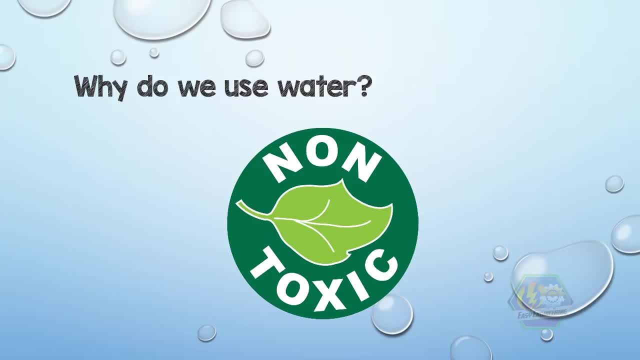 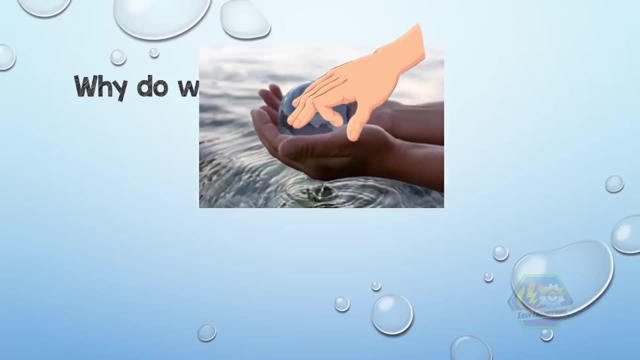 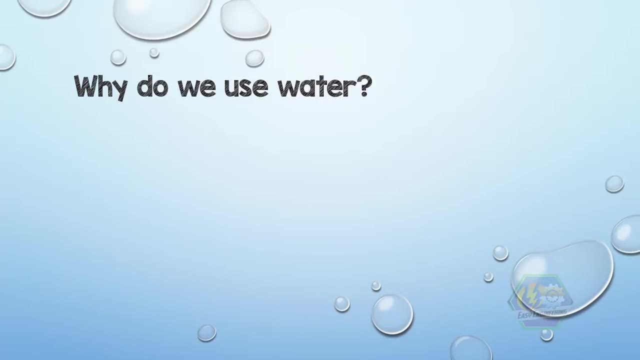 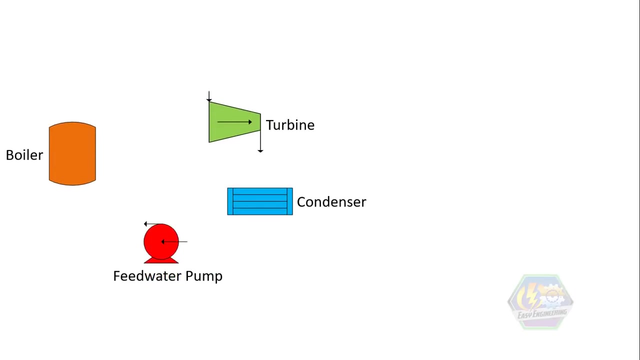 Well, simply because it is not toxic, not reactive, highly abundant, low cost and good thermodynamic properties. To make a Rankine Cycle we need four processes: Process 1 to 3 for the boiler, Process 2 to 3 for the turbine. 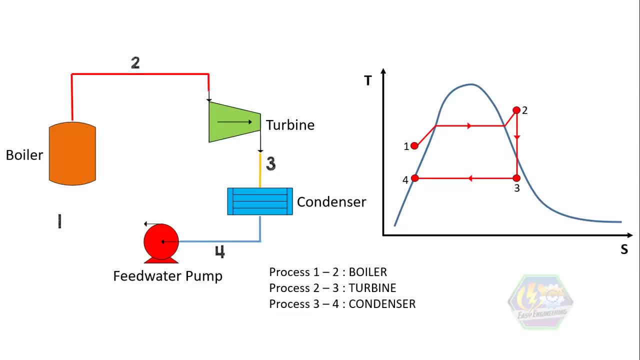 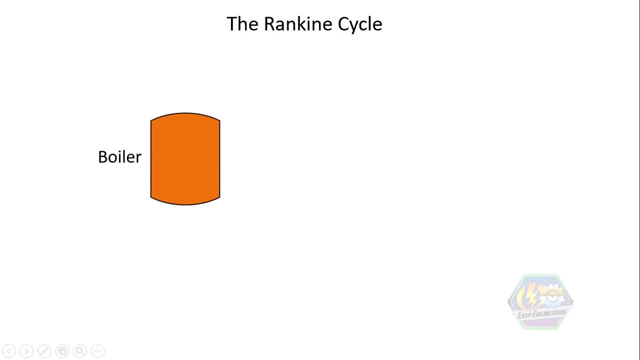 Process 3 to 4 for the condenser and, finally, Process 4 to 1 for the pump, And that is what we are going to discuss for the next part. Okay, so let's get this started. For Process 1 to 2: boiler, these are the things that we need to remember. 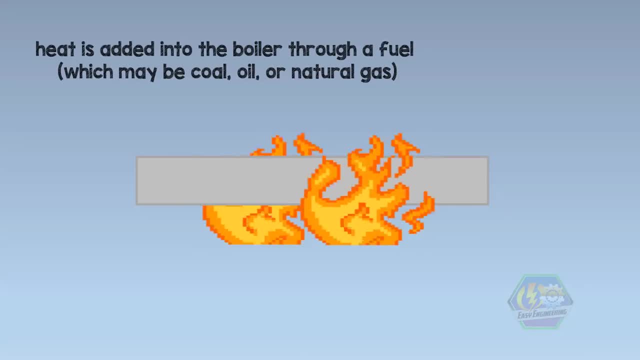 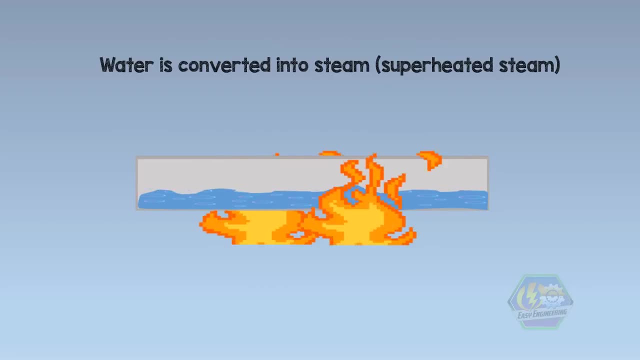 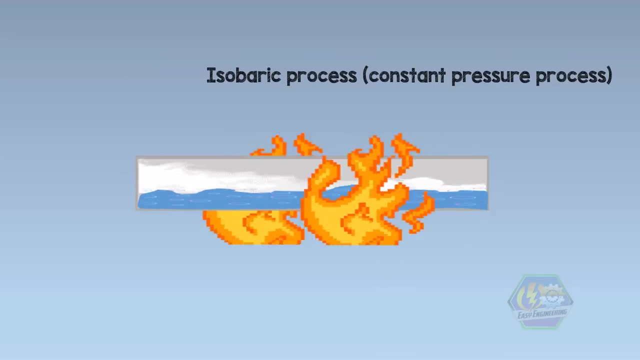 Since boiler is a heat exchanger equipment, a heat is added into the boiler through a fuel, which may be coal, oil or natural gas. Here, water is converted into steam or superheated steam. This is an isobaric process or a constant pressure process. 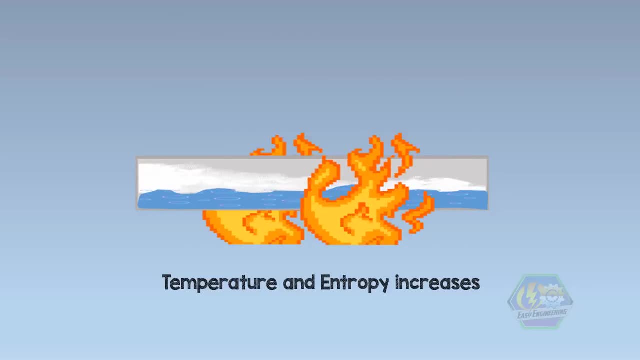 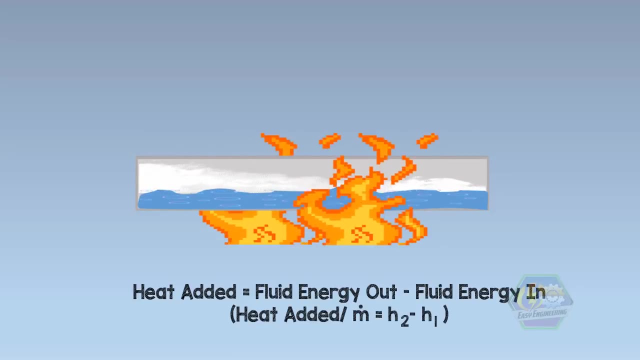 The temperature and entropy for this process increases, And we can solve the heat addition by using the formula: if added equals fluid energy out minus fluid energy in or enthalpy out minus energy in. For the boiler, Note that this equation is formed by using a mass and energy rate balance. 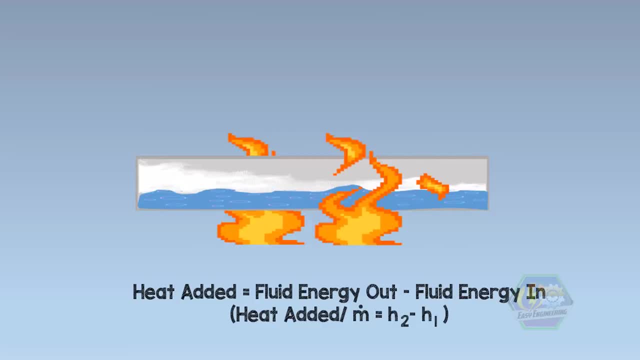 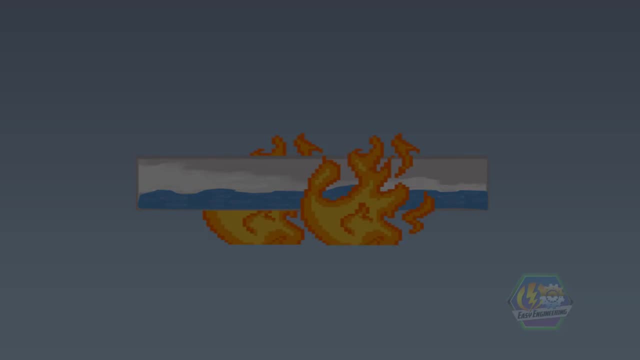 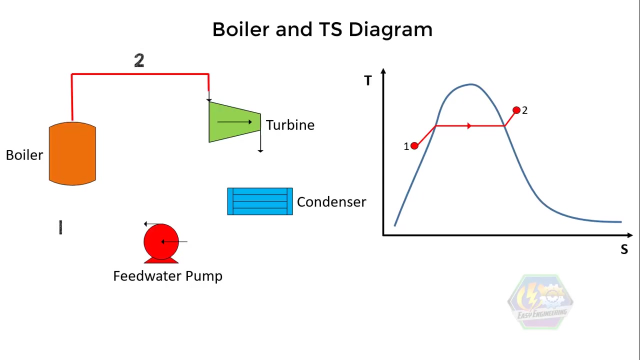 for a controlled building at steady state, neglecting pressure drop. So those are the important things that you should remember. with understanding the boiler process, Now steam can be used in the next process, which is the process of 2 to 3 turbine. 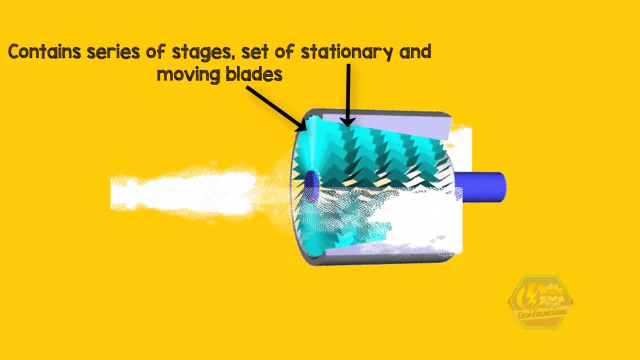 Turbine is a work generator equipment. It contains series of stages or set of stationary and moving blades to perform its function By using the steam. work is generated through the expansion of vapor, which may then be converted into electricity through generator. Compared to the previous process, 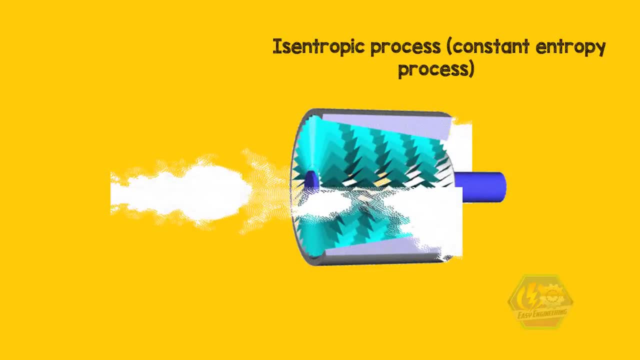 here, since we have an equipment that involves work, isentropic process or constant entropy process is used. This is assumed. Yes, it is assumed, because in real world there is no such thing as ideal. On this process, the temperature and pressure decreases. 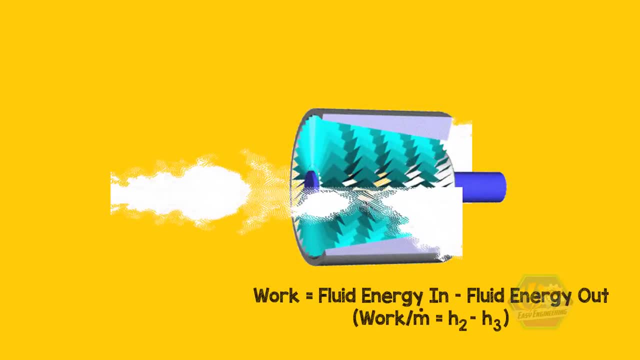 And the formula for the work is fluid energy in minus fluid energy out, or the enthalpy 2 minus enthalpy 3.. Note that equation is formed by using a mass and energy rate balance for a controlled bullion at steady state, neglecting heat transfer with the surroundings. 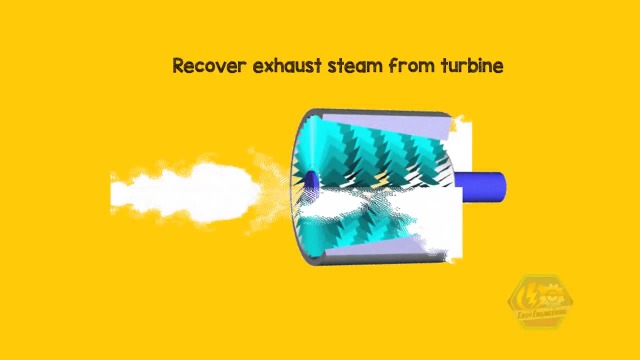 Steam is now already exhausted, and so we need to take it back again to the boiler. But there is no pump that can pump steam, so we need to convert it first into water through condensation. So this is where our next process comes in. 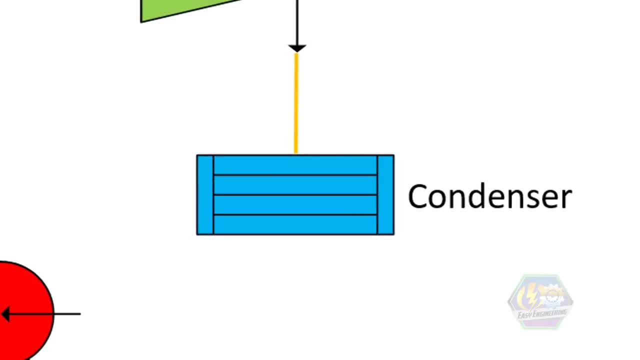 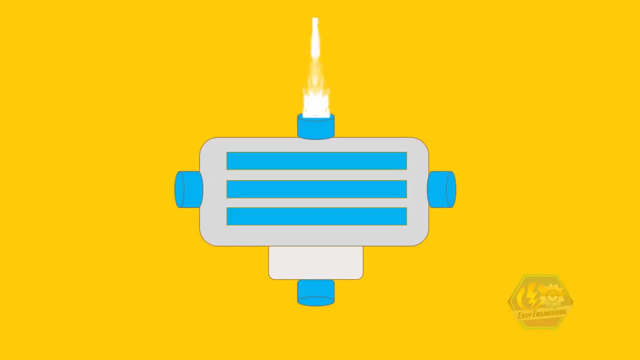 Process 3 to 4 Condenser. In order to condense the steam, a heat rejection must occur. Most of the power plants utilize the seawater as a cooling medium to cool down and condense the steam. Condenser consists of tubes to accommodate the heat transfer of steam and cooling water. 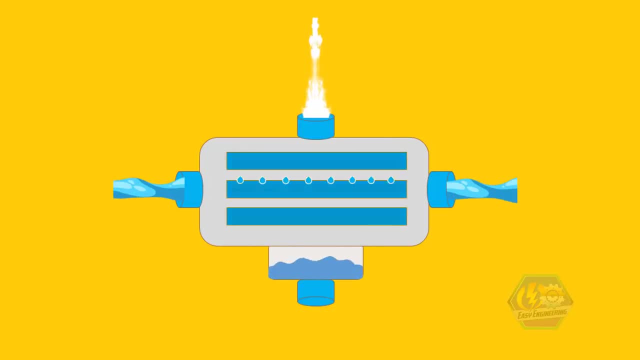 where cooling water is in a separate stream. This is a heat exchange equipment, so we assume that this is an isobaric process or a constant pressure process. The entropy decreases and the quality of the fluid changes until it reaches a saturated liquid state. 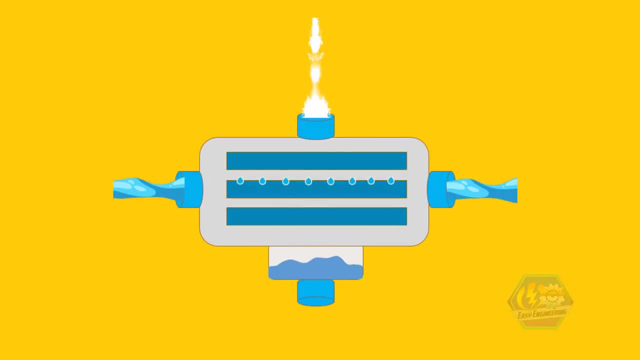 so from steam to liquid, The equation is: heat rejected equals fluid energy in minus fluid energy out, or enthalpy 3 minus enthalpy 4.. Note again that this equation is formed by using a mass and energy rate balance for a controlled bullion at steady state. 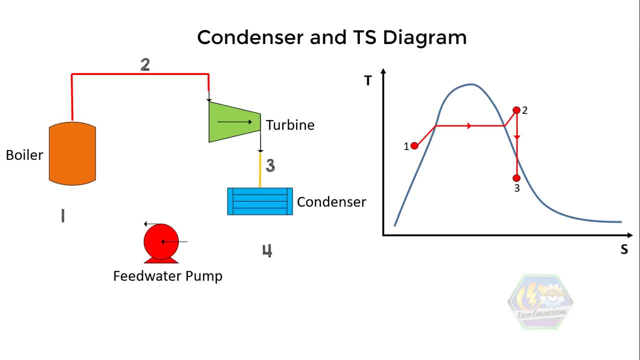 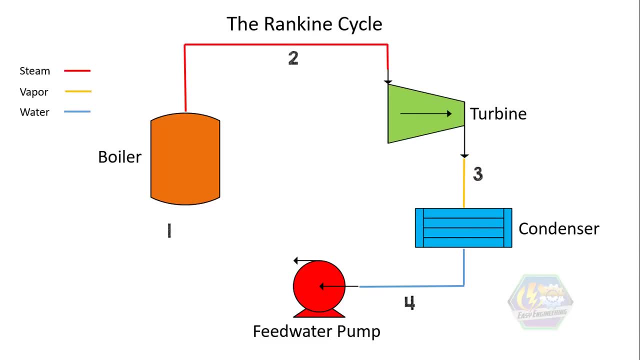 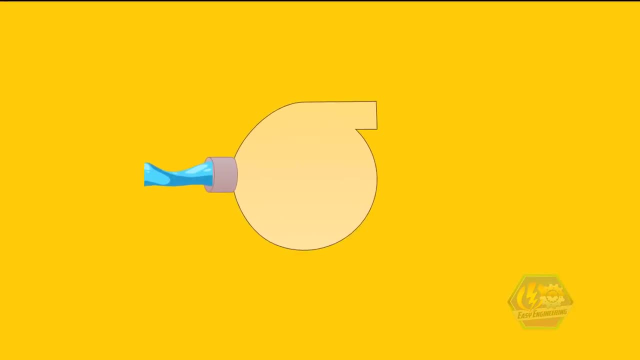 neglecting pressure drop. Last process is process 4 to 1 pump. Pump's main purpose is to convey and introduce back the condensed steam to the boiler. Here work is needed. That means work is negative. Some plants name this pump as boiler feed pump. 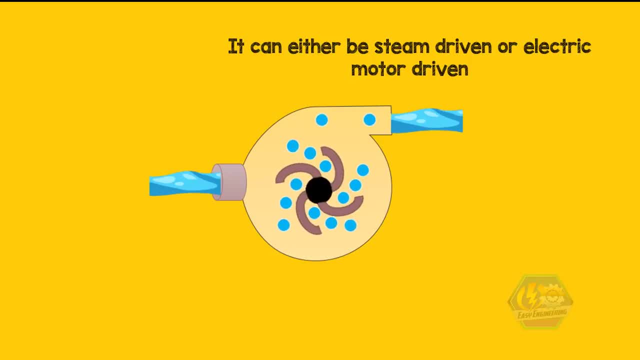 and it can be either steam driven or electric motor driven. Again, since this is a work involved equipment, we assume that this is an isentropic process or constant entropy, The temperature slightly increases and the fluid is in a sub-cold region in the TS diagram. 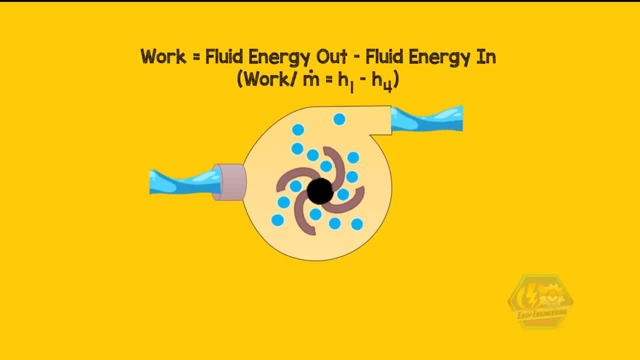 The formula for the pump is: work equals fluid energy out minus fluid energy in or enthalpy 1 minus enthalpy 4.. Fluid energy out or enthalpy out is greater than the enthalpy in, as the pump have imparted energy to the fluid. 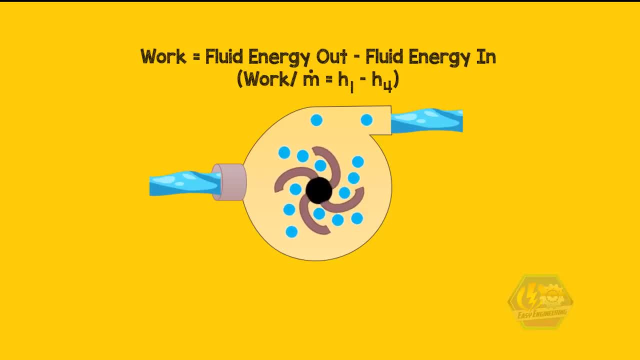 Note again that equation is formed by using a mass and energy rate balance for a controlled bullion at steady state, neglecting heat transfer with the surroundings. And one more important thing: please remember that the pump has the highest pressure in the whole cycle. 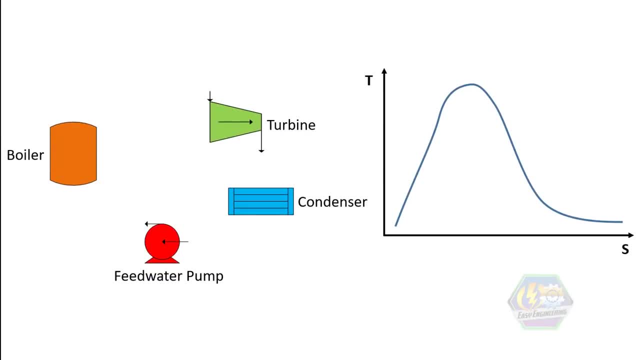 Okay, so let's have a recap. Starting from the boiler, we convert the liquid water into steam, Introduce it into the turbine to generate work, and then we condense it into the condenser and pump the liquid water back to the boiler through a high pressure pump.